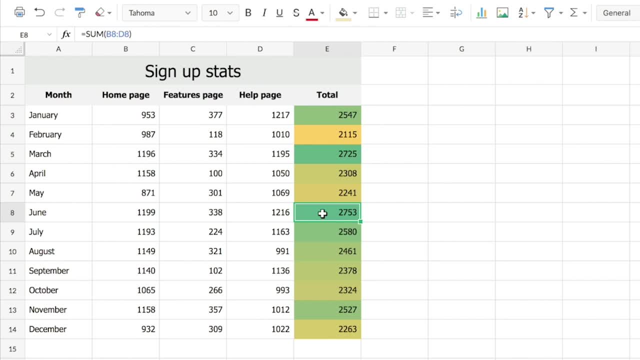 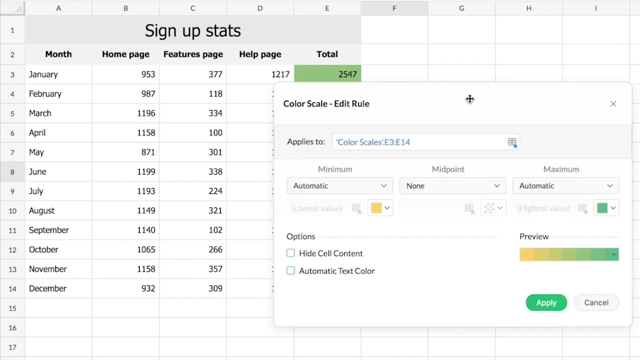 green background set, while the other cells have the shades. so this makes it easier for me to know which month performed well and which did not. now let's just open up the color scale dialog and see how the rules have been set. so this is the color scale dialog, as you can see the minimum and maximum values. 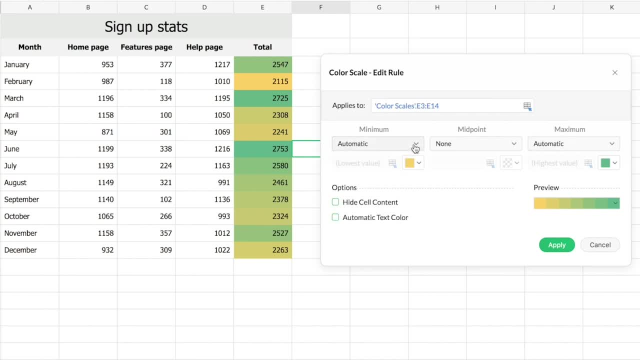 have been set to automatic, because I chose from the menu directly. if you want, you can even customize these minimum and maximum points, and they can also be in terms of number, percentage formula or even a percentile value. so the whole sheet also gives you the option to choose the color for your color scale. so 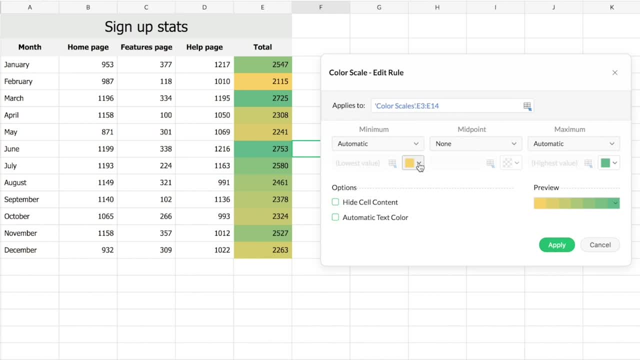 you can even customize those colors in the scale. and additionally you can find two other options here at the bottom. so one is to hide the cell content. so one says check string, which is project check. then these three options will say: click on that and you will see a black layer warning. you see that the background. 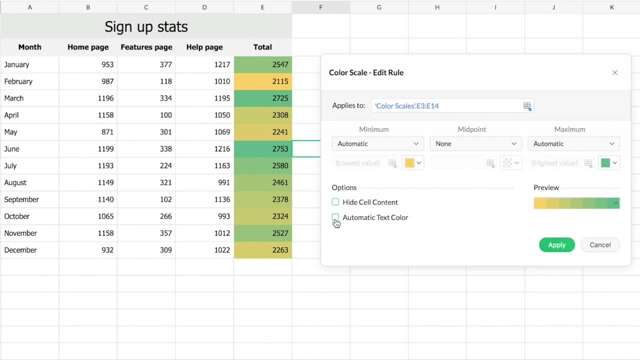 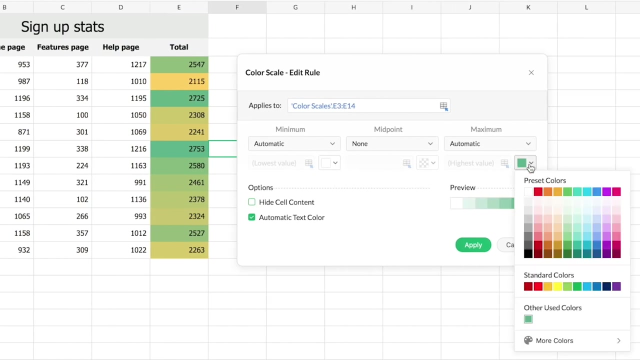 is white and you can also know which color is the white layer in this product. so once this option is checked, the cell values in this range will be hidden and only the cell background color will be displayed. and there's another option here for automatic text color. so once I click on that, the cell font color will 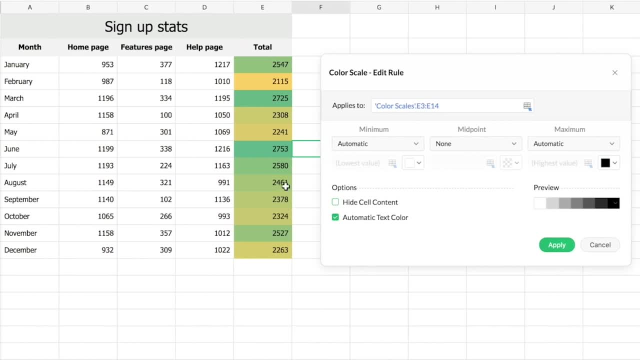 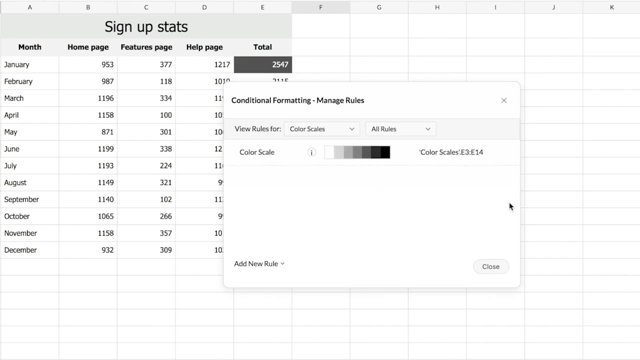 change based on the cells background color. so to demonstrate that I'll just colors in this cell range are all black. so now that I've set the background color from white to black, let's see how this font color changes based on the automatic text color option. so I click on apply now. 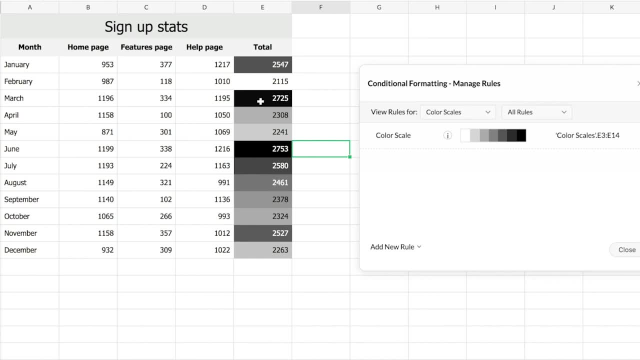 and, as you can see, those cells with the dark background color have a lighter font color. it is, the cell with a black background has a white font color, and so on. so this option increases the readability of cell values when these background colors are applied. so that's all about color scales in Zoho Sheet.